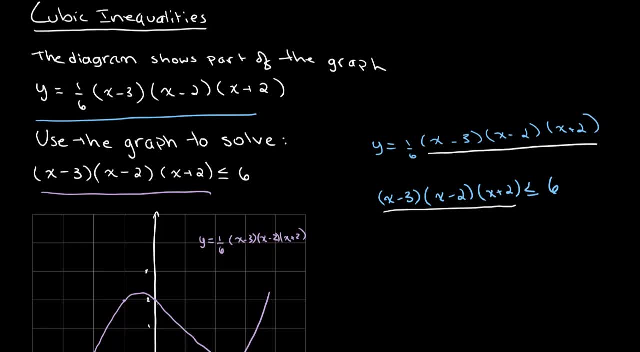 x minus 3 times x minus 2 times x plus 2.. The only real difference is the 1 over 6.. So we want to get this equation, or our inequality, to match this whole entire equation that we have over here. 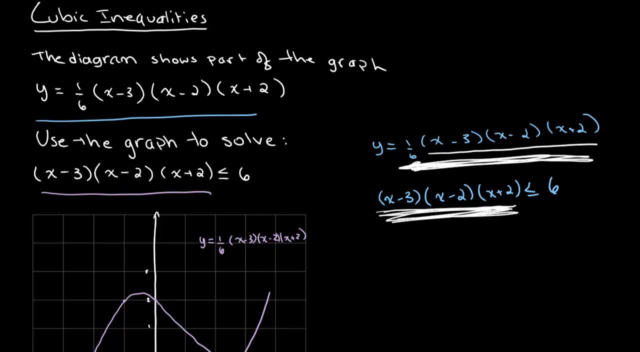 So how do we do that? What we can do is we can just multiply this by 1 over 6.. So we get 1 over 6 times x minus 3 times x minus 2 times x plus 2.. Now you see, by multiplying it by so times 1 over 6, by multiplying it by 1 over 6, we 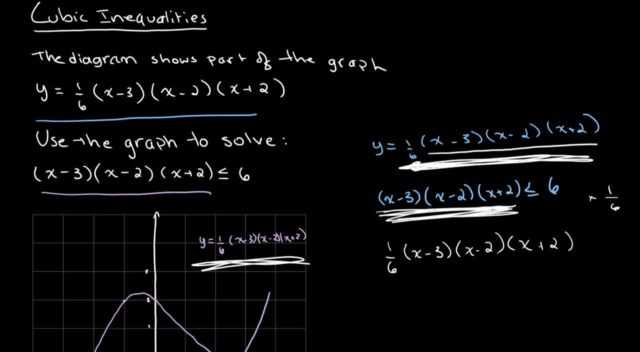 made it match. So this is our graph, or the equation represented inside of our graph, And this is less than or equal to 6 times 1 over 6.. So we get 1 over 6 times x minus 3 times x minus 2 times x plus 2 is less than or equal. 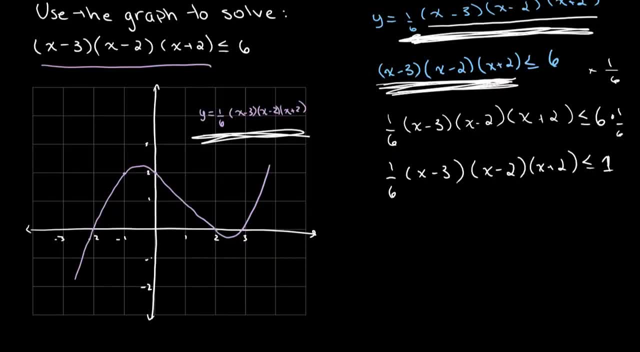 to 1.. So now our inequality over here matches the equation represented inside of our graph. So how do we find our answer now? Well, we want to find all of the points where this equation is less than or equal to 1.. So we find the line y is equal to 1 in our graph. that would be right over here going. 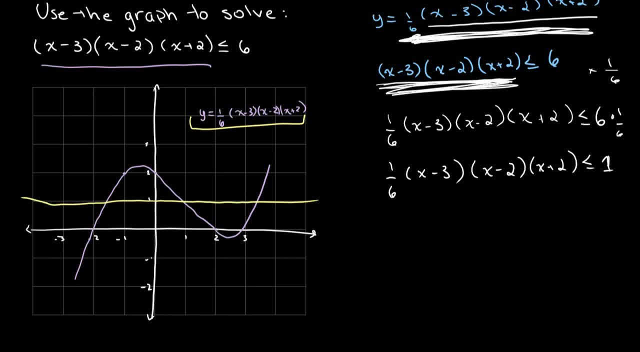 like this, And we want to find all of the places where our equation is less than or equal to it. So we see that, from this point going down, Okay, So our graph is less than or equal to 1.. And from and in this part of our curve, our graph is also less than or equal to 1.. 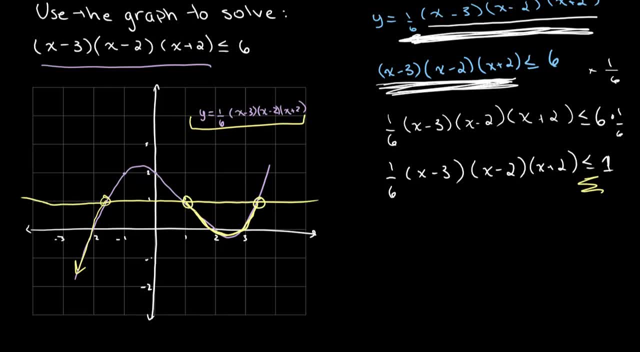 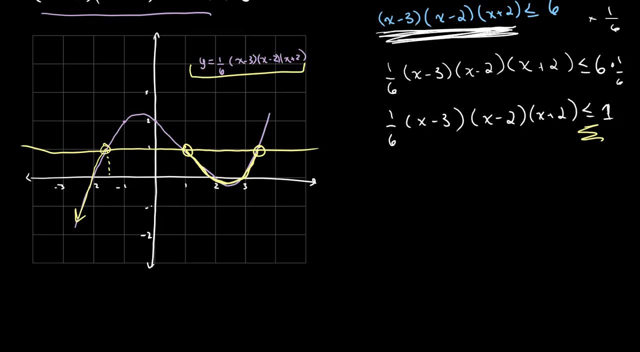 So that's between this point and this point. Now we just need to represent that as an inequality. So this point over here is about negative 1.6.. So x can be less than or equal to negative 1.6.. So that represents this part of our graph, or all of the values going in this direction.